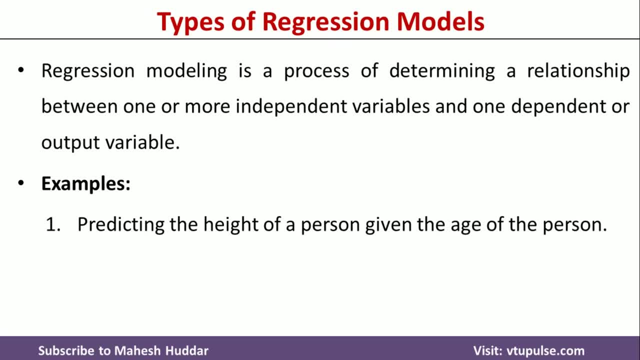 height. that is, the dependent variable means height depends on age in this case. We will take one more example. In this case, we want to predict the price of a car given the car model, year of manufacturing mileage, engine capacity and so on. The meaning of this one is the: 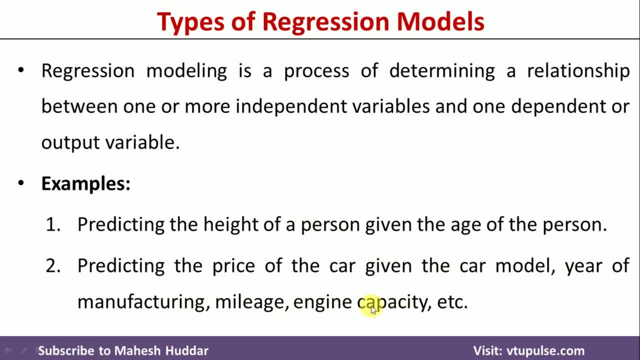 car, model, year of manufacturing, mileage, engine capacity are independent variables. If you know these particular values, we want to predict the price of a car, that is, the output variable or a dependent variable, in this case, The process of finding, or you can say that getting- the relationship between these independent 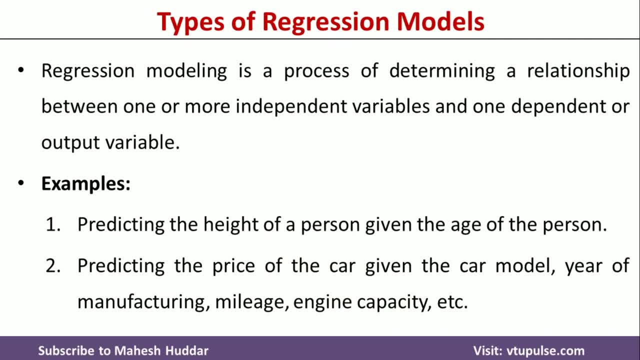 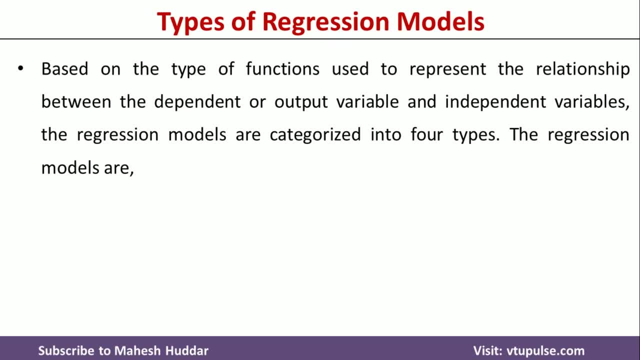 and dependent variable is nothing but a regression model, in this case Based on the type of functions used to represent the relationship between dependent and independent variables. the regression models are categorized into four types. The first one is simple, linear regression. second one is multiple regression. third one is polynomial regression. fourth one is logistic. 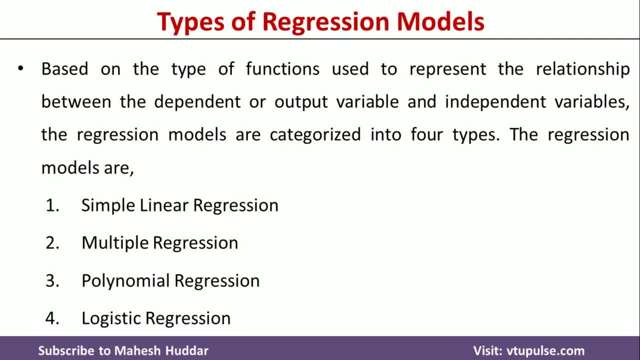 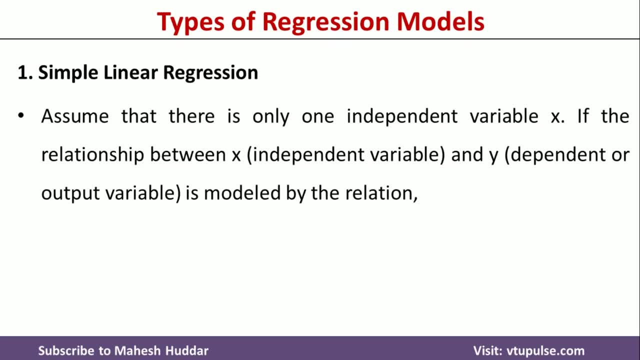 regression. Now we will try to understand each of these models in detail. Simple linear regression model: Assume that there is only one independent variable, that is X, and the relationship between this x, that is the independent variable, and y, that is dependent or output variable, is modeled. 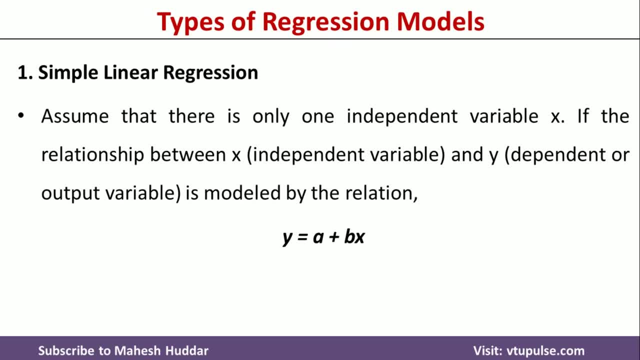 by the relation y is equivalent to a plus bx, then this relationship is called as simple linear regression model. So in this case we have one independent variable, that is x, and we represented this relationship like y is equivalent to a plus bx. If you know the value of 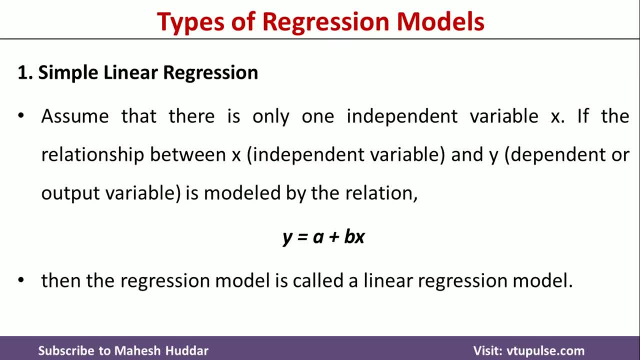 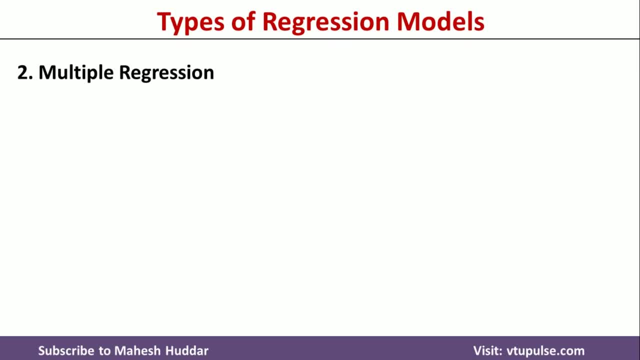 x, we can easily predict the value of y in this case. So this is a simple linear regression model in this case. Now coming back to the second one, that is, multiple regression model, in this case there are multiple independent variables. let us say that x1, x2 till xn are. 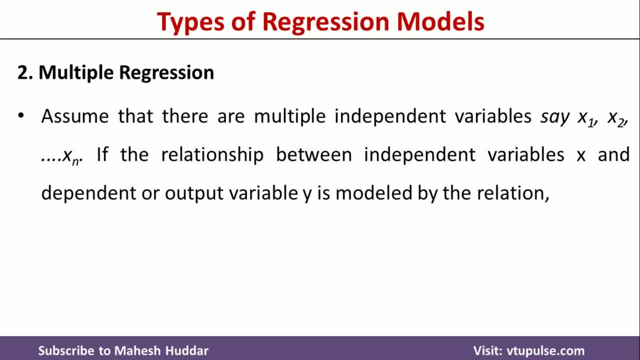 the independent variables, and we want to find the relationship between these independent variables and the output variable. Let us say that it is represented by this equation: like y is equivalent to a0 plus a1x plus a2x, dot, dot, dot an xn, Then this kind of relationship is called as multiple regression model In multiple regression.